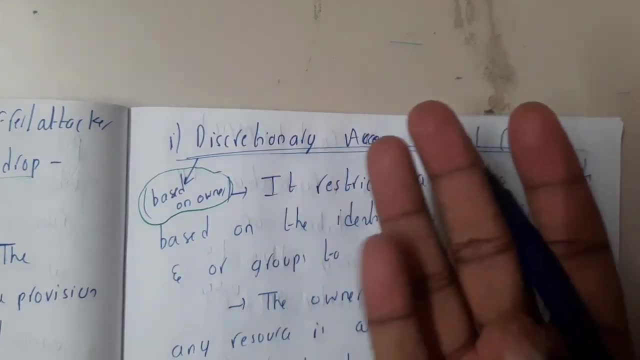 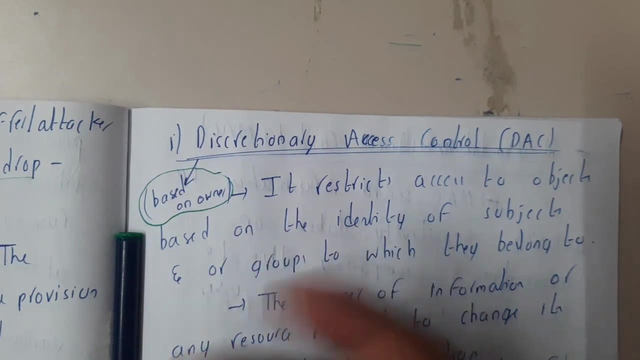 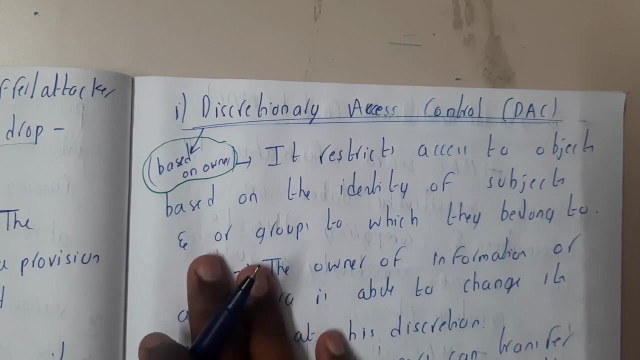 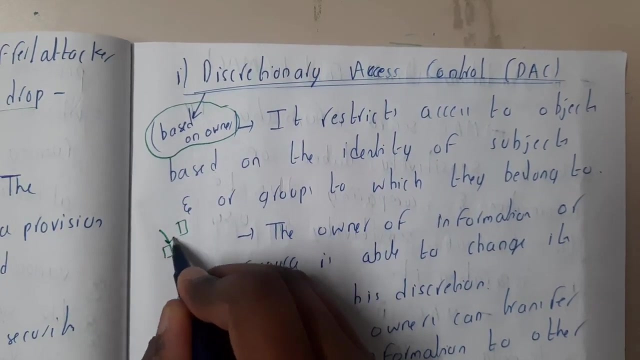 So every power is in his owner's hand, So he can change those rights to you like anyone he can do. He can do anything on the data, right? So, because he's the owner, right, Yeah, so he will be having the permissions. Okay, so he's restricts access to objects based on identification of subjects and or group to which they belongs to. So assume that you are a company owner and there is a project, guys. you got Okay, so this project. there is abstract and all those things, guys, So the project has been given. So there is some. 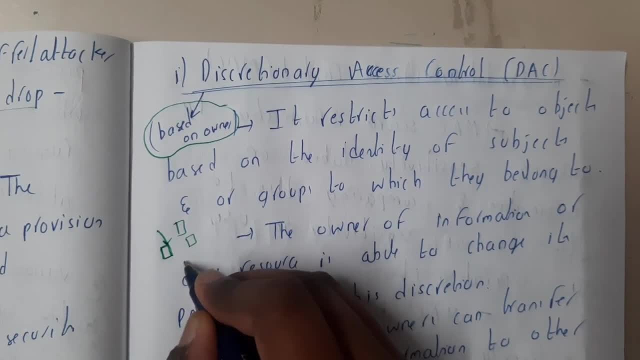 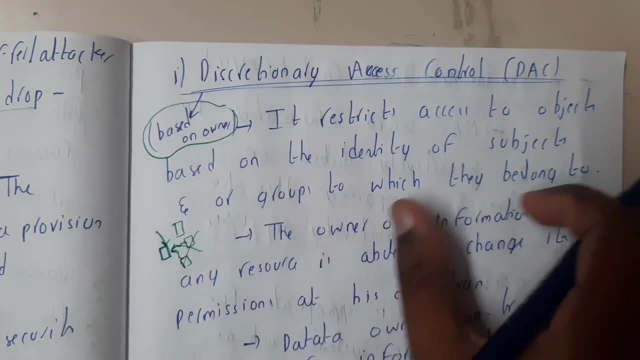 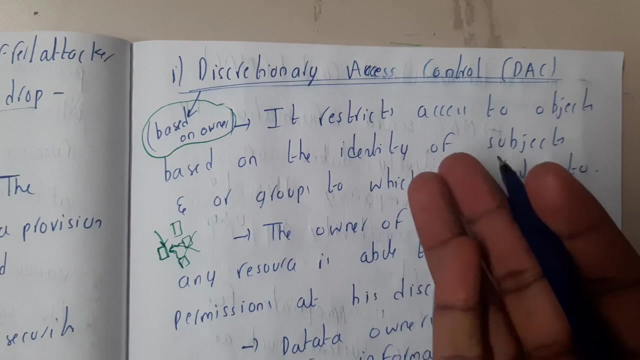 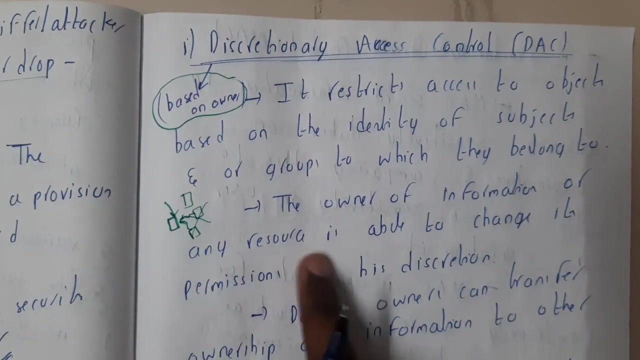 branch in your company, who is for finance and who is for marketing. So is there any need for them to have access for this project guys? No right, Yes, So in the same way, only the group who needs or identified subjects or identified users, like project managers, the project employees, the team members for them, only should be given access. So those things will be managed here. Okay, so the owner of information or any resource is able to change the permissions at his instance. So if he wants to avoid, 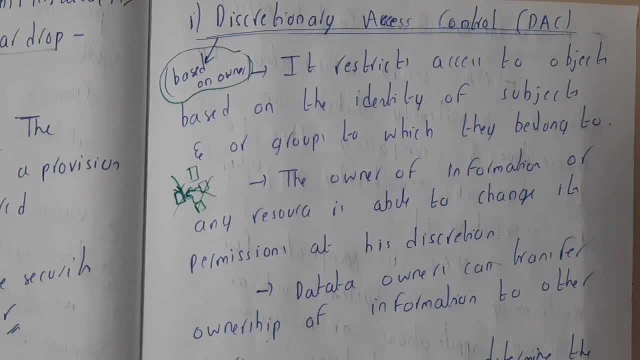 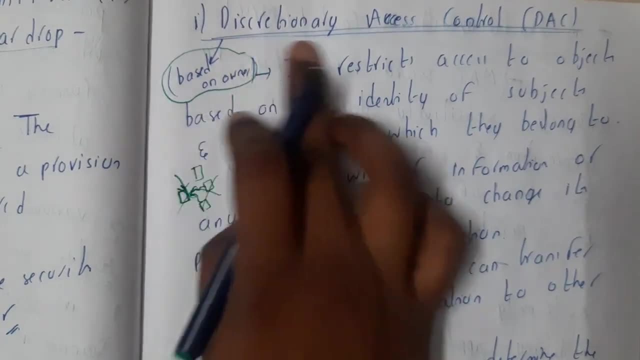 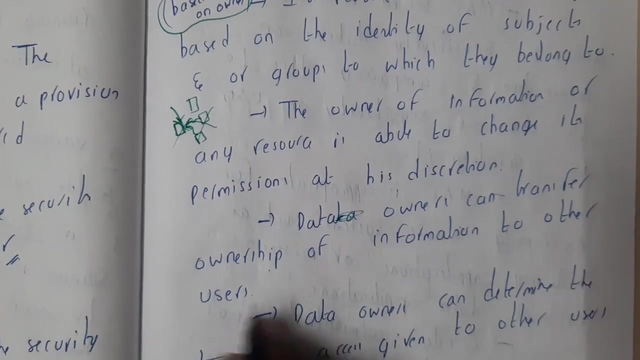 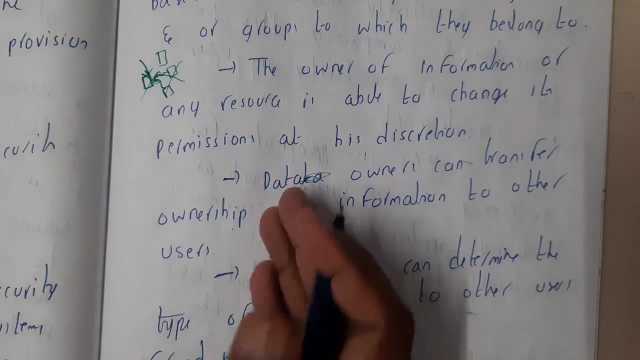 even for this project members also, only for team leaders and project managers. if he wants to you, he can do that. There is no issue with this, because there is a free to use. That is nothing but DAC. That is nothing but discretionary access control right, Yes, So data, Okay. so data owner can transfer ownership of information to other users. So basically, if he's going off for a leave or some kind of thing, he can transfer. Sorry, he can transfer the leadership to some other, So that 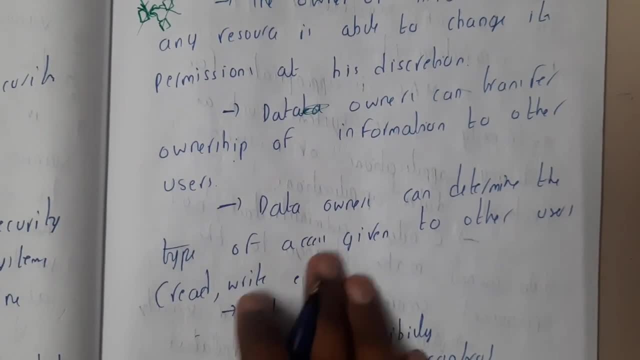 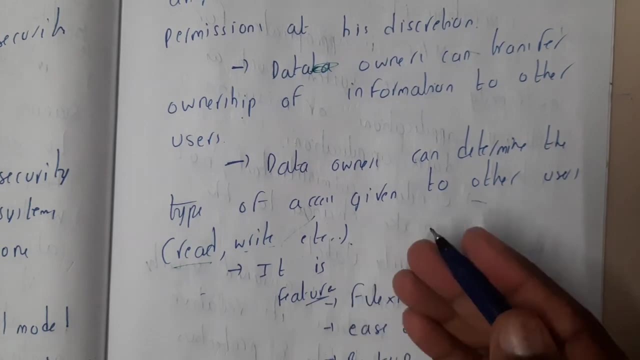 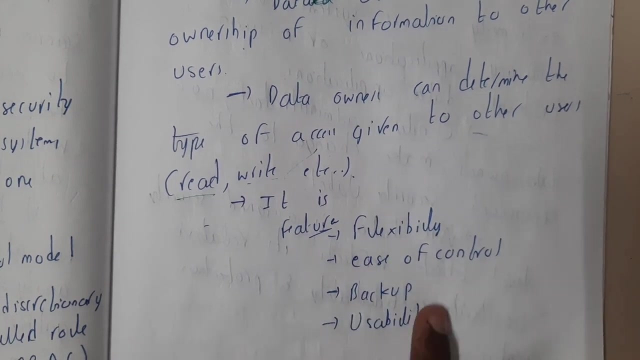 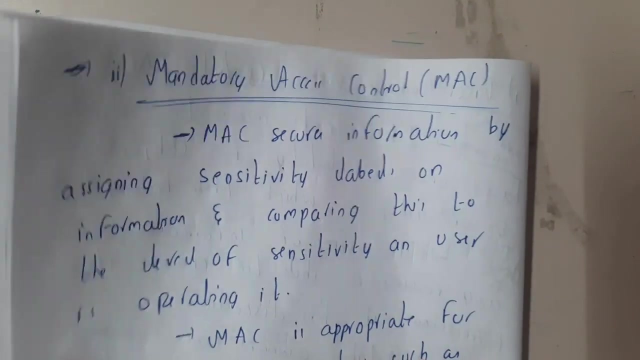 other will be taking care of the team till then, right? Yes, So the data owner can determine the type of accesses given to other users So they can read or they can rewrite, or they can update, or they can modify or whatever they can do. Everything will be specified clearly, guys. Okay, so the futures of this is nothing, but it is flexible, easy to control, backups will be taken and it is usability. It is good for using, right? Okay. the second type is nothing but a mandatory access control. So a simple, strict version of the DAC is a. 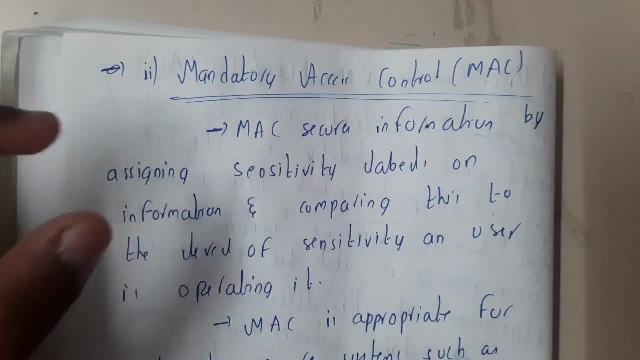 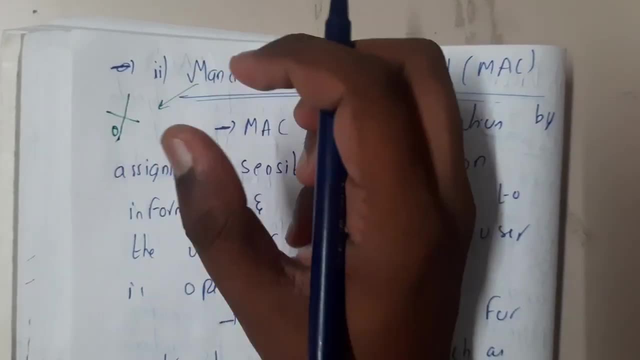 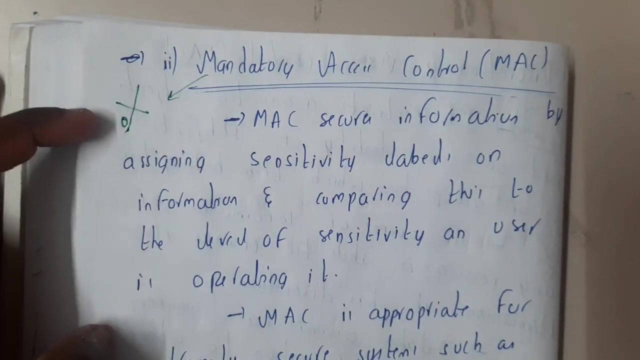 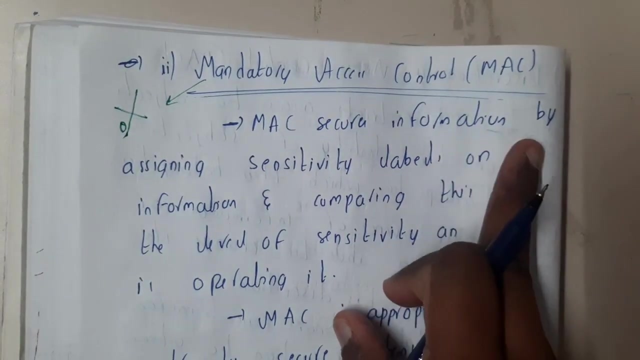 nothing but a MAC, guys, Mandatory access control. Okay, so here the trick is that even the owner cannot do any kind of operation. So once the file or once the data has been given, okay, so the administrator is only the one who can do any kind of changes, guys, because he's the king, right? The administrator- he's going to have all the rights. Yes, So Mac secures information by assigning sensitive labels on information. and comparing this to: 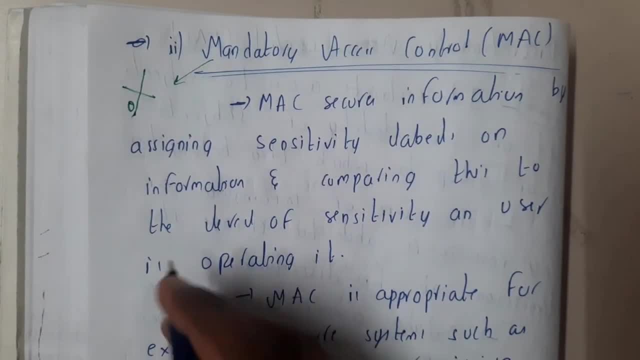 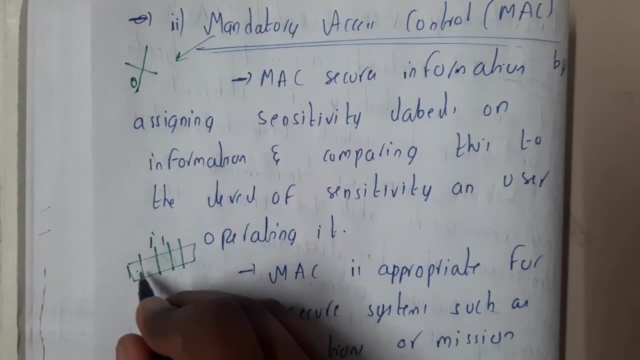 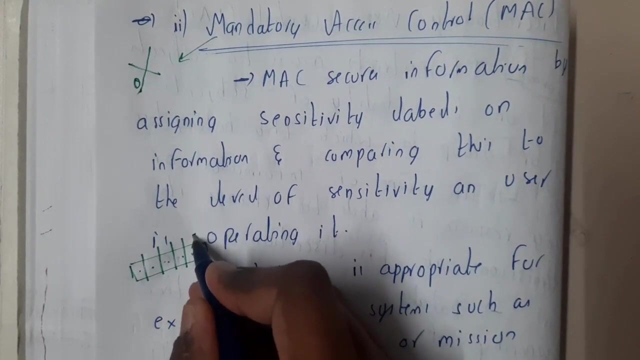 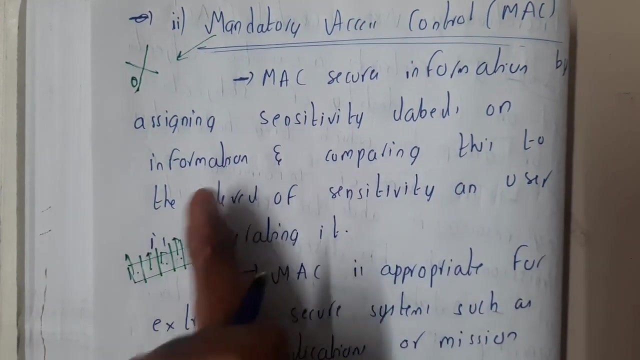 the level of sensitivity on user is operating. So basically, here we will be dividing the whole spectrum into multiple parts, guys. So if you ask me an example, I'll be dividing into 1, 2, 3,, 4, 5.. Okay so I think 1, 2, 3, 4, 5.. It's already 5.. Okay so the first part will be very low, low, medium, high, very high. So, based on its importance or based on its priority, I'll be dividing them and a few users will be in this part, few users will be in this part. the main leaders and everyone will be in this part. 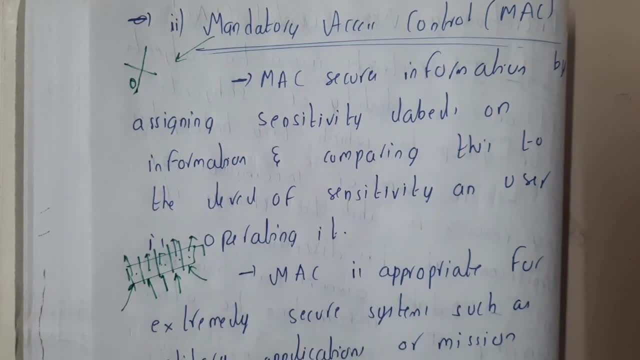 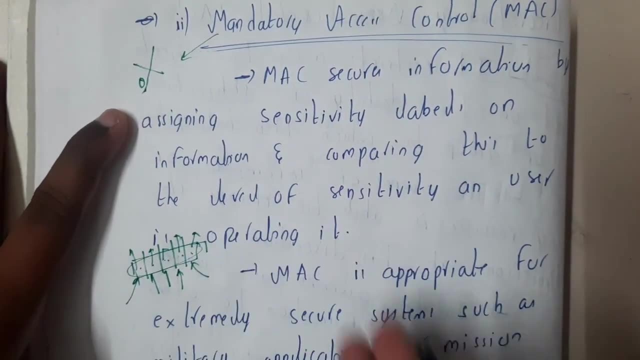 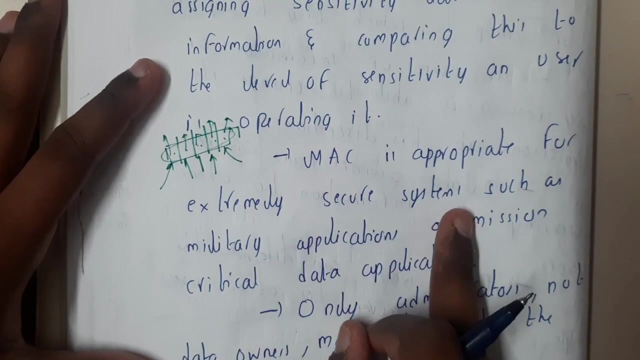 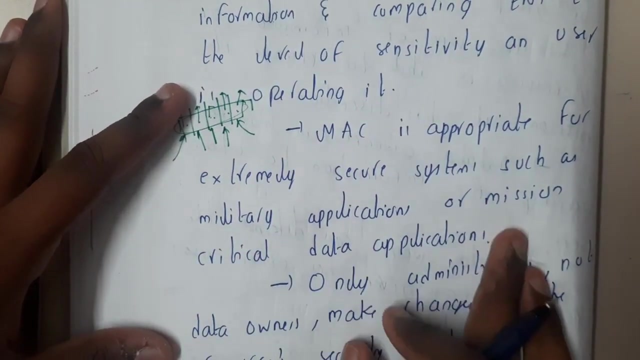 Like that. based on these sections, they'll be dividing and they can access the data. So this concept is given as a Mac guys and this addresses these changes, these position changes, and everything will be done by the administrator. Okay, yes, So Mac is operated for extremely secured systems, So here we are dividing into multiple segments. It's a bit complex, right? Yes, because our data is that much important, such as military applications or machine critical data applications. Okay, so who is having the permission? The administrator. So only. 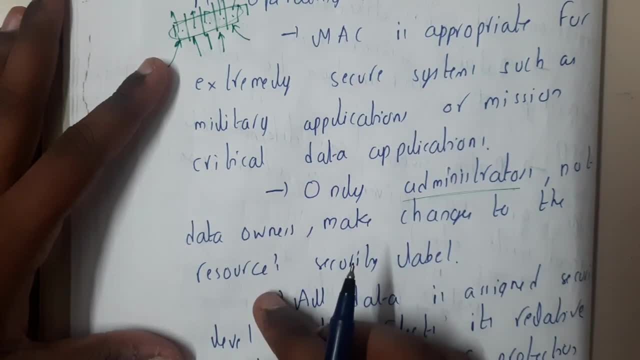 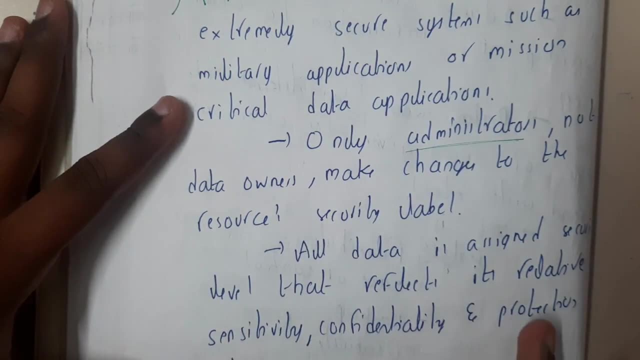 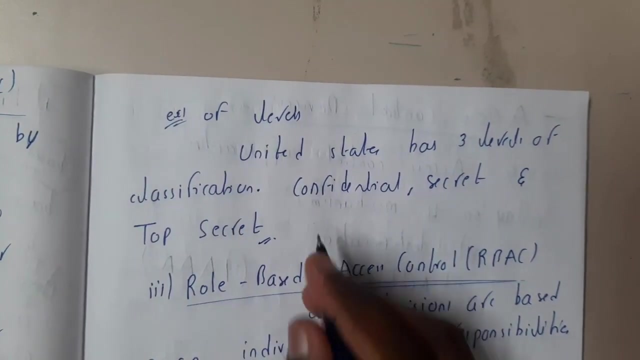 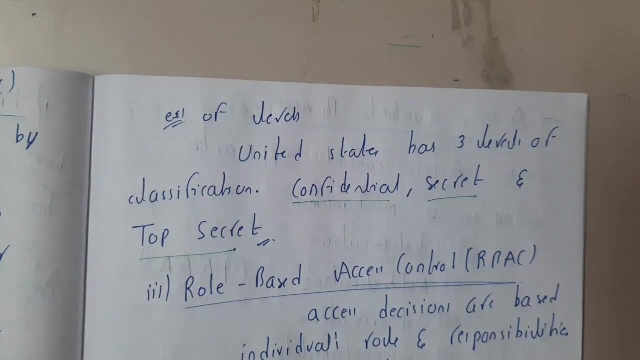 administrator, not even the data owner, make changes to the resources or even these access permissions. Okay so all data is assigned secure levels. that reflects its relativity security and all those things. Okay so here we wrote an example of US state 3 level classification. guys, They'll be having 3 levels in military. that is nothing but confidential, secret and top secret. Okay so, based on these levels, they'll be dividing the whole employees or the officers and based on their criteria, they will be accessing the data.